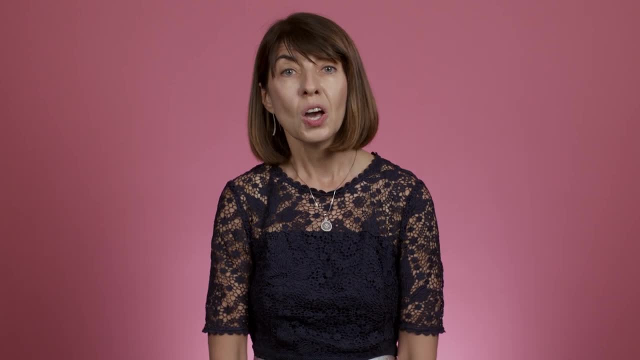 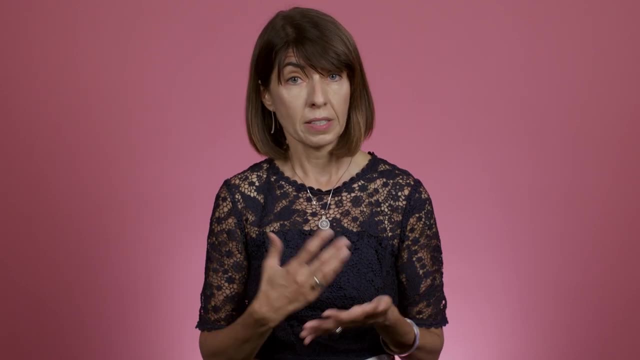 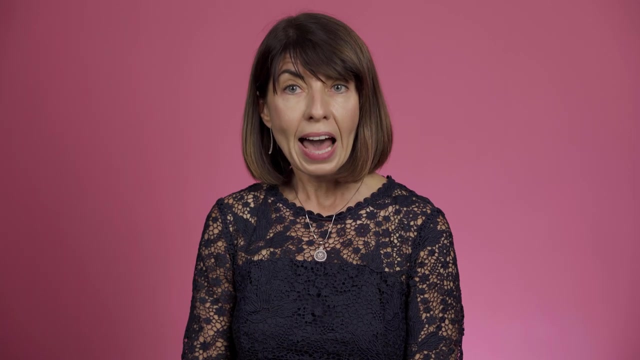 at a time when the dominant interaction style was the command line. In a command line interface, if the user wanted to use a command line to delete an item from the desktop, they would have to type a command like this one. There are several attributes that are essential to direct manipulation. 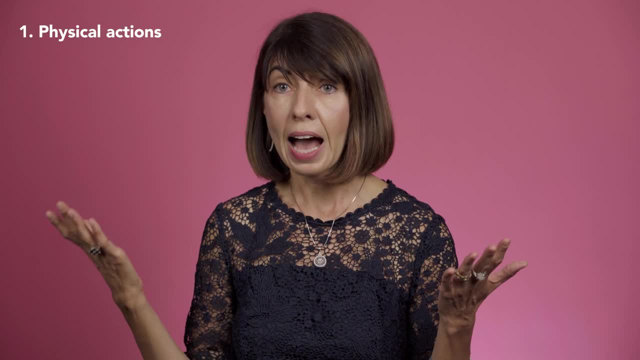 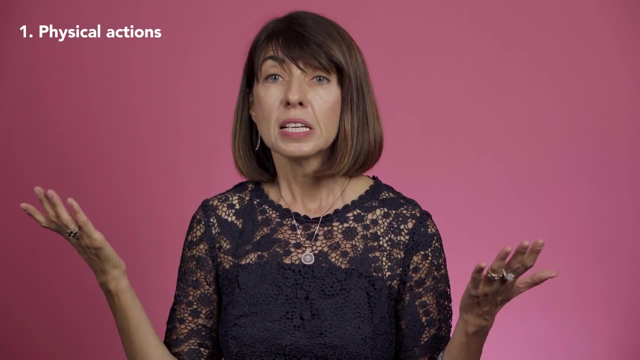 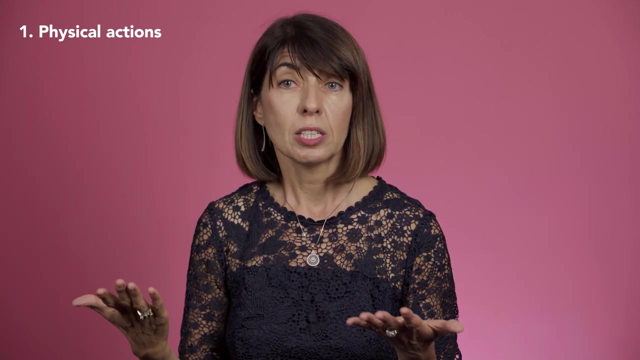 First, the interaction happens through physical actions like drag and drop or pinch open. Many of such physical actions are inspired by the real world. For example, drag and drop a file to move to the trash bin is very similar to this one, But if you want to delete an item from the desktop, you'd have to type a command like this one. 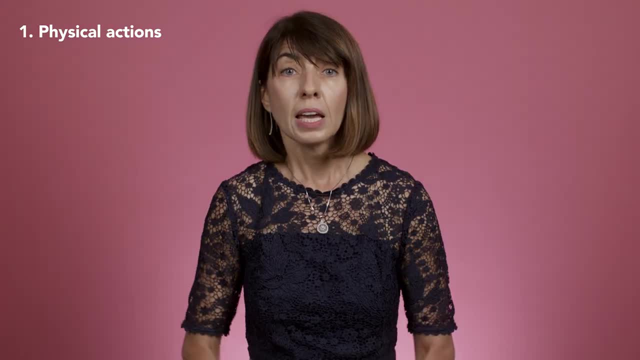 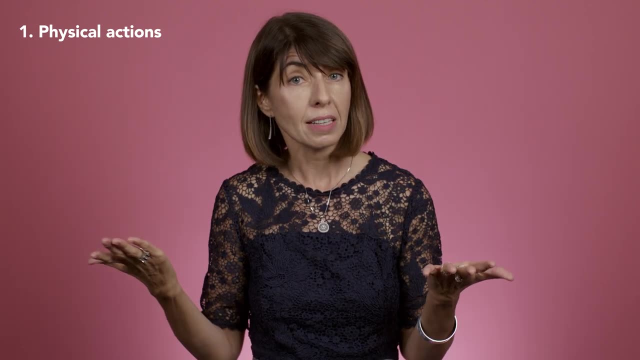 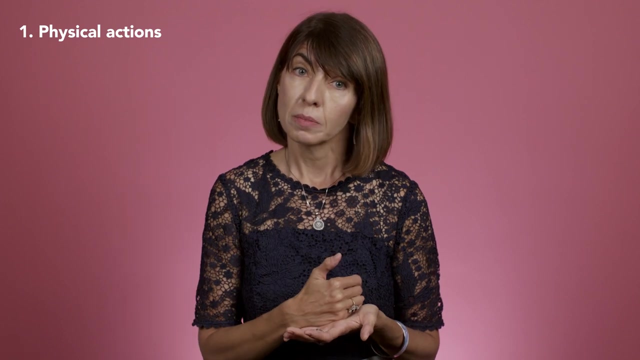 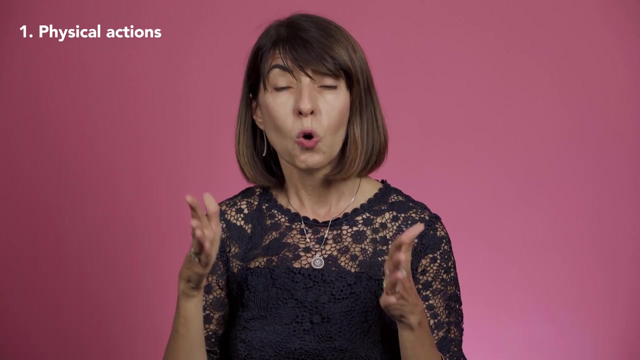 to throwing an object into a physical trash can. Interacting through physical actions means that the user does not have to remember the name of a command like rm for delete in our command line interface example, or the name of an object like the name of the file to be removed. We say that direct manipulation favors recognition over. 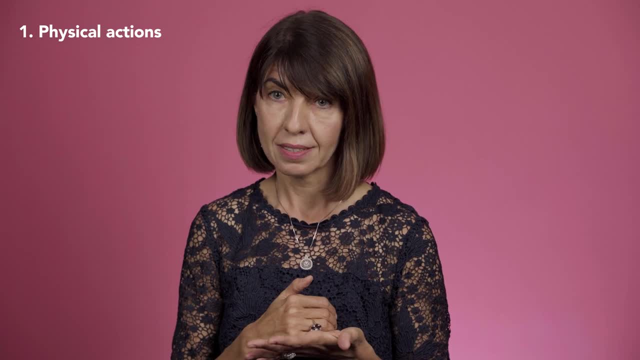 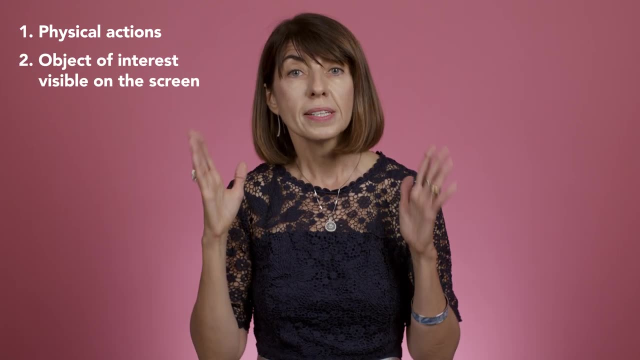 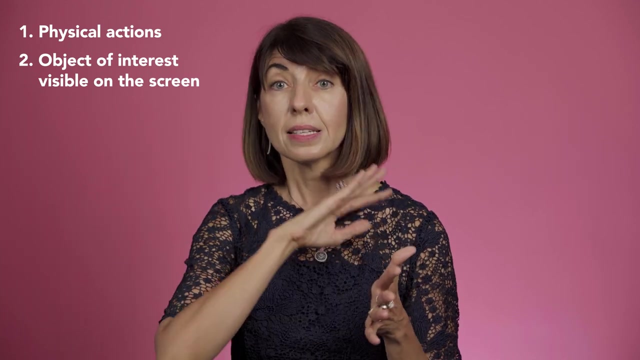 recall, which is one of the 10 usability heuristics. Second, with direct manipulation, the objects of interest are always visible on the screen. For example, users can see the file on the desktop and then they can see it disappear once it gets dropped into the recycle bin. 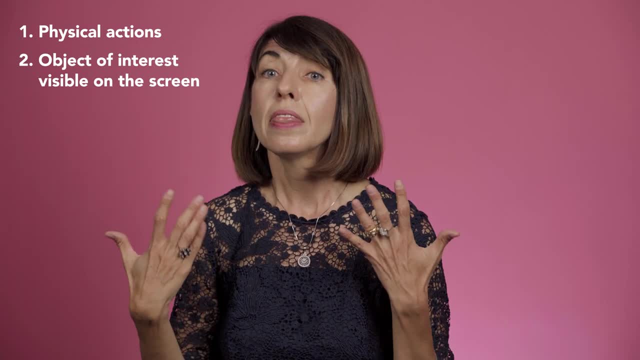 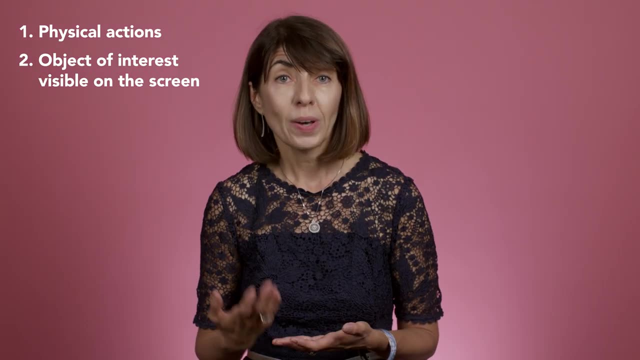 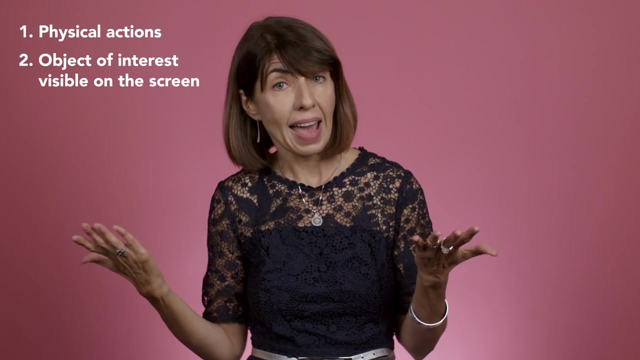 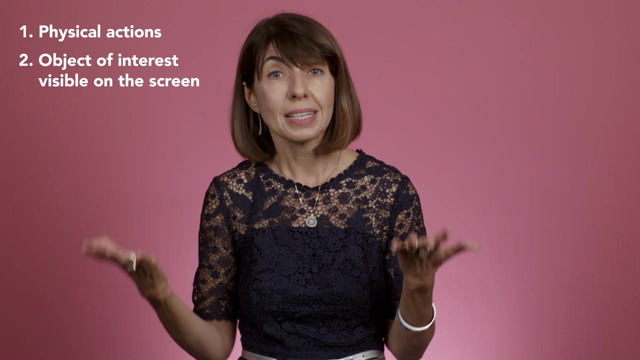 Thus direct manipulation satisfies another usability: heuristic visibility of systems status. Because of it, it's easy to check whether an action has been completed successfully, whereas with a command line interface you must perform some other action, such as listing the content of the folder in which the file used to be, to make sure that your action was successful. 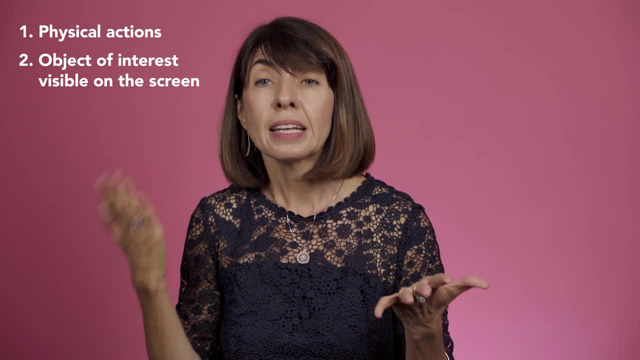 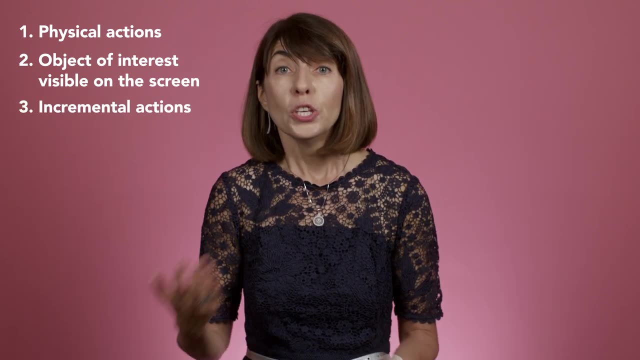 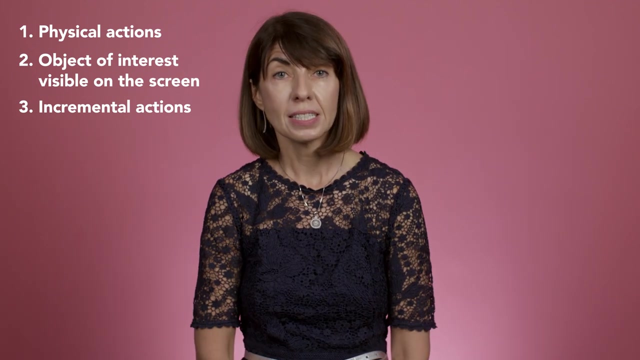 If an error has been made, it's easy to detect it and correct it right away. Third, direct manipulation actions are incremental. You can perform only one basic action at a time. That can be sometimes perceived as a disadvantage, especially when there are many such actions that need to be performed as part of a bigger task.